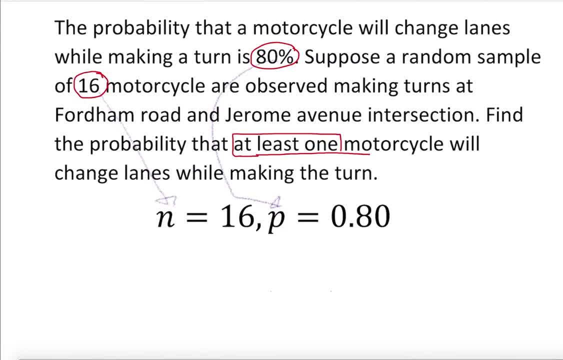 Like that. Okay, So what does this at least 1 mean? At least 1 really mean is probability of X greater than or equal to 1.. That means- well, I'm going to actually put down here to the right side: So in this case is 16 of them: 1,, 2, 3,, all the way up to 16.. So at least 1.. Remember, if this is also 0 here, So at least 1.. 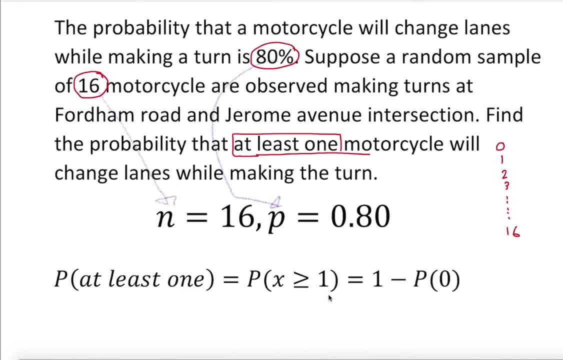 If we can somehow say probability of everything should be 1. And I somehow subtract the 0 here as you clearly see. So I can actually get at least 1.. So best you know, at least 1.. So 0 is in this case, is also 1 probability here. So 1 minus. this is what is not happening here. At least 1 means what. 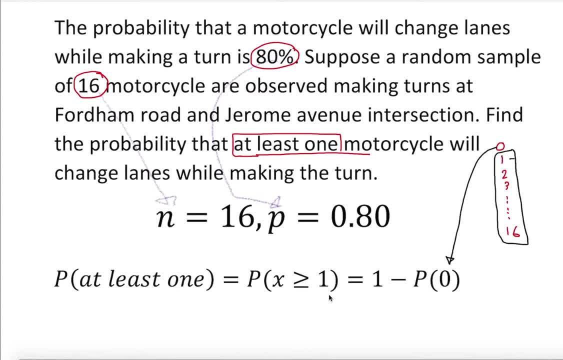 1.. 1 or more, 1 or more, 1 or more. You go all the way up. That's what at least 1 means: 1 or more. So I can just subtract 1 minus probability of 0. I get that. Or I can just add all of these Probability of 1 plus probability of 2 plus probability of 3 and so on. This is going to be too much work, Okay, So we don't want to do that actually. So probability of at least 1 is always better. If this is probability of at least 1, then it's better. 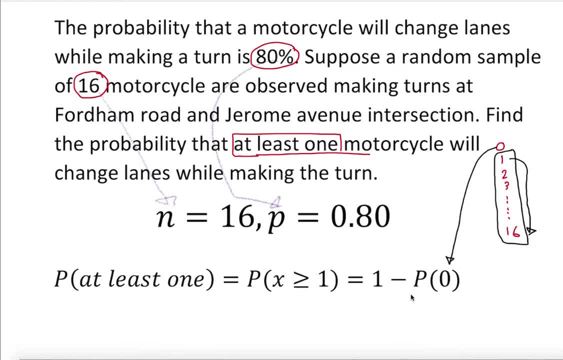 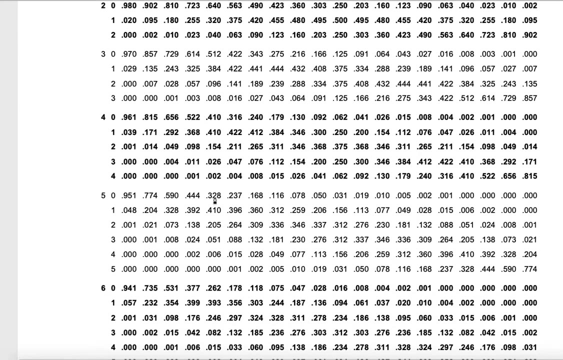 Okay, At least 2.. So we can say 1 minus probability of 0, minus probability of 1.. That's how we can actually play with. So 1 minus probability of 0. What is probability of 0?? Let's take a look into the. So we have 16. Then phi is 80. And we do 0. So 16, phi is 80. So let's go with binomial probability here, We go with the 16. So if you go 16.